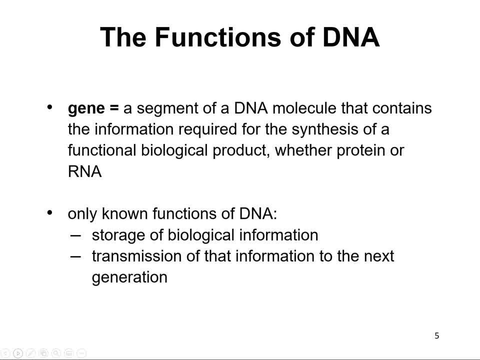 A gene is just a segment of DNA that has the information, And that information is what makes it possible for a gene to be able to produce a functional biological product. That could be a protein or that could simply be an RNA. I say simply: RNA is anything but simple. You'll see that. 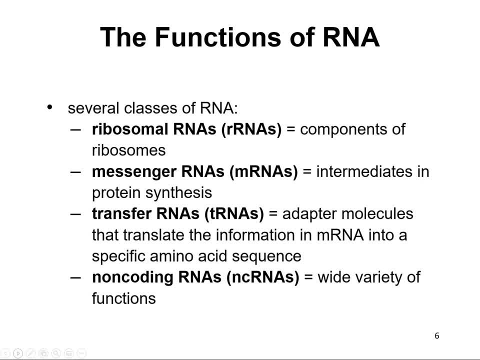 There are several classes of RNA. We've got ribosomal RNA or rRNA, which you'll be responsible for. knowing all of these little abbreviations for RNA, It'll just help you out a lot when you're reading. Ribosomal RNA is a component of the ribosome. 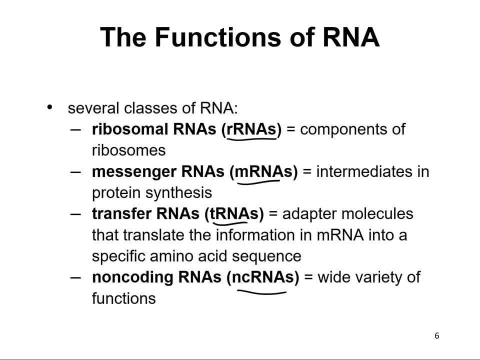 And the ribosome is responsible for taking the messenger RNA and translating it into protein. Messenger RNA, mRNA, is the intermediate between DNA and protein, So messenger RNA is formed. it's also called a transcript, so an mRNA transcript, just because it is a transcript of DNA. 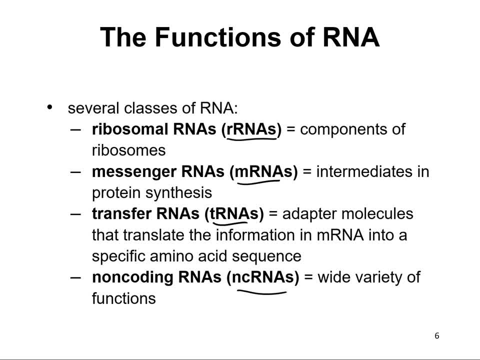 That has the code for making the protein. So it's going to bind to the ribosome and interact with tRNAs, the transfer RNAs, And these are adaptor molecules that bind to amino acids. So it recognizes a three-letter code on the mRNA and it brings along with it the correct amino acid. 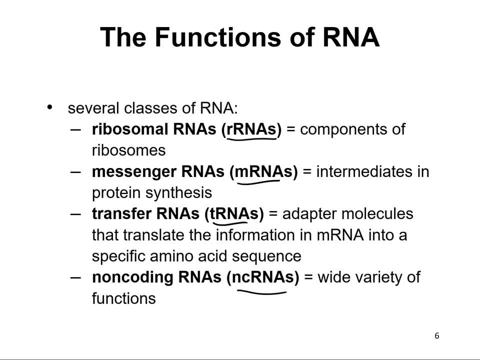 So that that polypeptide strand can bind to it, So that that polypeptide strand can bind to it, So that that polypeptide strand can bind to it, So that that polypeptide strand can be formed. 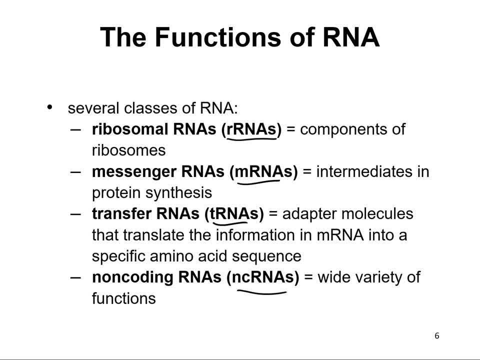 So you've got the tRNA recognizing the mRNA, And then you've got on the other side, you know, this growing polypeptide chain. We're going to cover all of this at the end of the class when we talk about, you know, RNA and DNA metabolism. 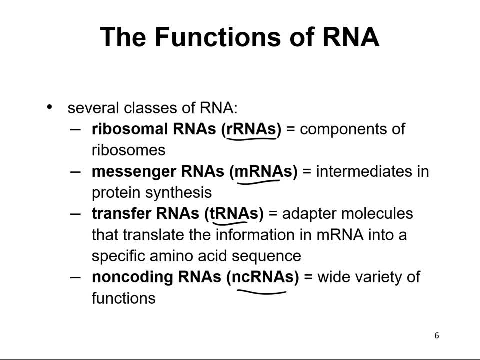 So don't worry about knowing that. for now, These are probably things that you've already encountered in all of your biology, And we're just kind of refreshing, And we're just kind of refreshing, And we're just kind of refreshing at this point. 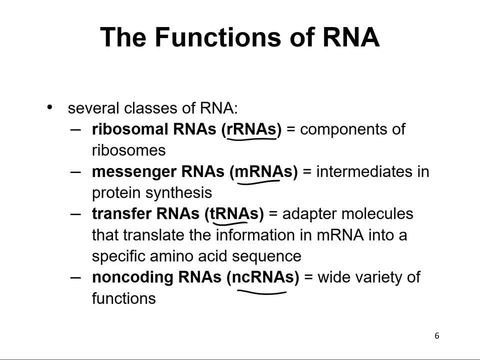 The last one that you may not have heard a whole lot about in your biology classes is non-coding RNA, And these have a wide variety of functions, Everything from the spliceosome, which helps to splice messenger RNAs and make them into what they're supposed to be before they are translated into protein. 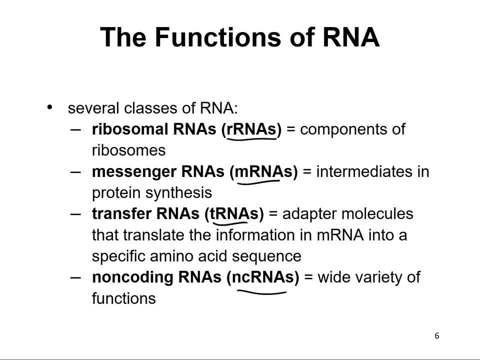 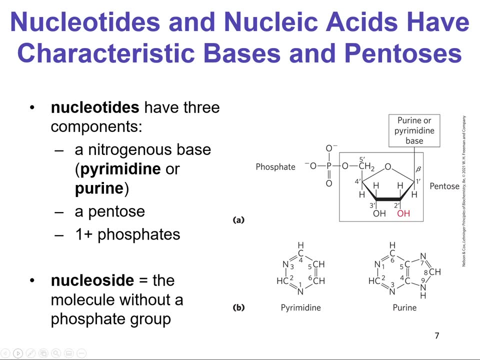 to silencing different sections of the genome. so all kinds of things. non-coding RNAs are really interesting. they have a wide variety of functions. nucleotides and nucleic acids have characteristic bases and pentoses- pentoses, throwback to chapter 7. so all of this builds all the. 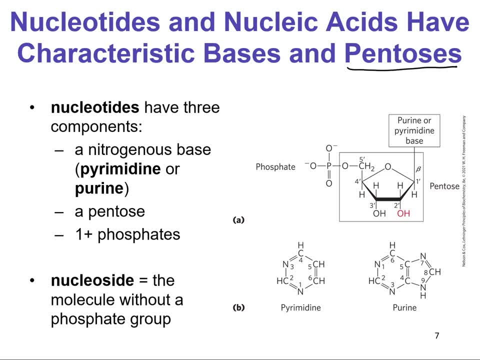 vocabulary when we're talking about sugars. some of that's going to apply to our conversation about nucleic acids and nucleotides. so nucleotides have three components: there's the nitrogenous base, there's the pentose to the sugar and then you have at least one phosphate. okay, so nucleotide has phosphates. that 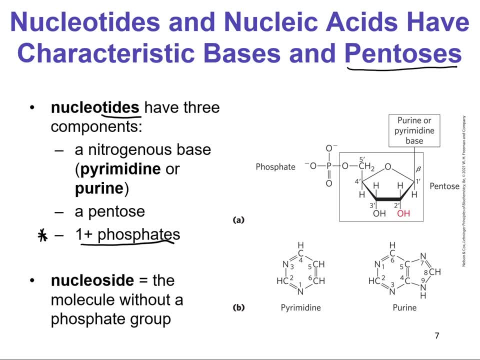 nitrogenous base is either pyrimidine or purine. pyrimidines are. I think about it as this way, because you'll need to know what the base is and then you'll need to know the difference. pyrimidine, long name, little molecule. so it's like opposites. 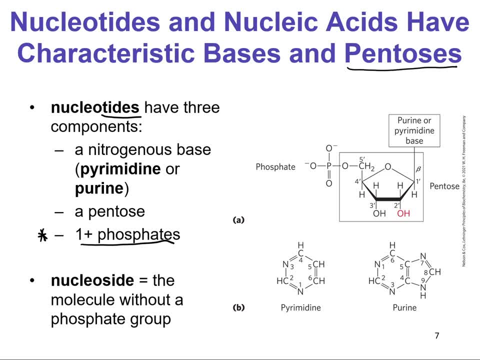 the purine actually has the two ring structure and we'll talk more about this, specific nucleotides and nucleosides in a second nucleoside we're talking about the nitrogenous base plus that pentose sugar, no phosphate. so know the difference between nucleotide and nucleoside. 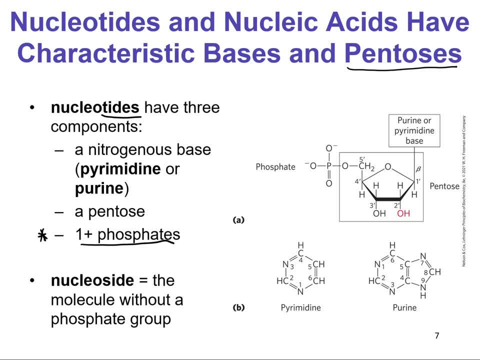 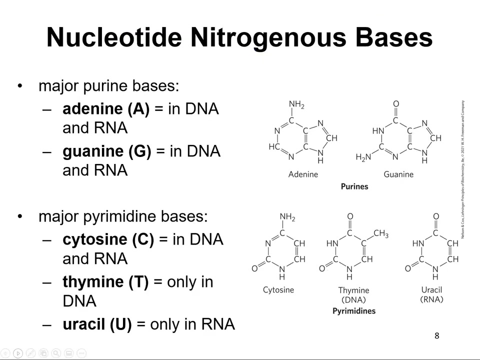 you'll also want to pay attention, as we talk more about nucleotides, nucleosides, to this two prime position here. this is the determining factor for whether you're looking at DNA or RNA, if you're looking at deoxy versus just ribose. okay, these major purines and pyrimidines. you'll need to know these, recognize them. recognize. 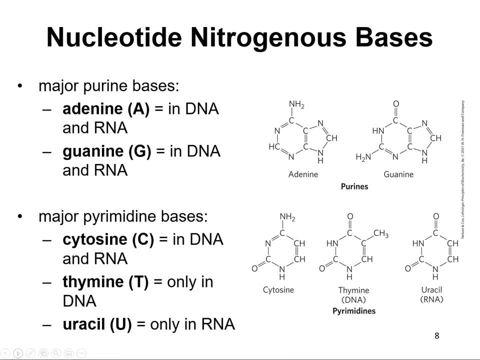 them in their nucleotide state and nucleoside state: a, G, C and T. those are all in DNA. thymine is only in DNA, that's the T. uracil replaces thymine in RNA. so you'll need to know which ones are in which molecule, and the answer is: everything is in DNA and RNA except for thymine. 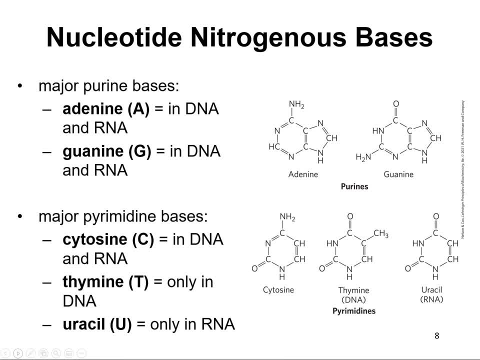 and uracil. so thymine is DNA, uracil is RNA. you'll need to be able to recreate these purines and pyrimidines, so be able to draw the difference between these two. so you'll need to be able to draw the difference between these two. so you'll need to be able to draw the difference between. 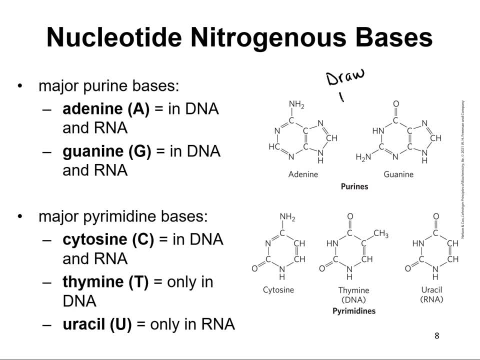 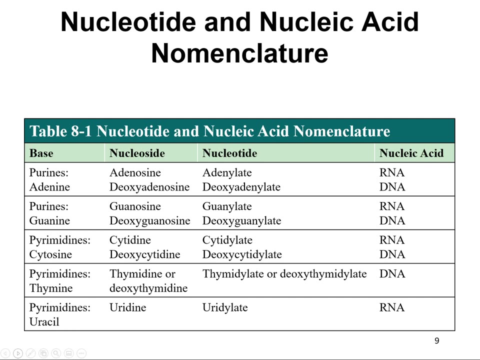 them. I'm not gonna make you responsible for drawing nucleotides and nucleosides, but I do want you to be able to draw the purine or the pyrimidine. this table gives you some help with nomenclature. so if we're talking about purines, we've got adenine and 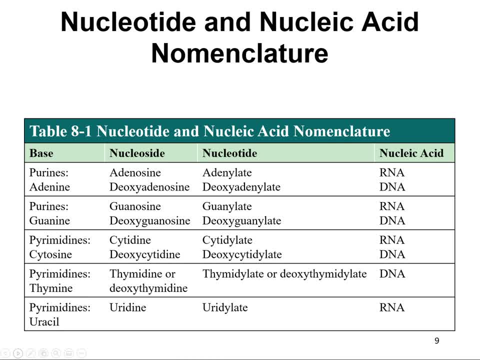 guanine. the nucleoside for RNA is adenosine, for DNA it's deoxyadenosine, so that two prime hydroxyl group is gone. there's no hydroxyl group there. same goes for the comparison of RNA and DNA, for all of these, the exception being looking at thymine and uracil. so if we're talking about thymine, 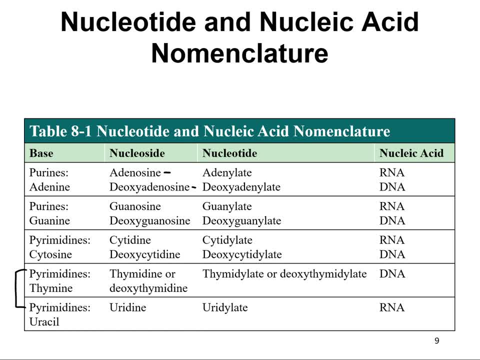 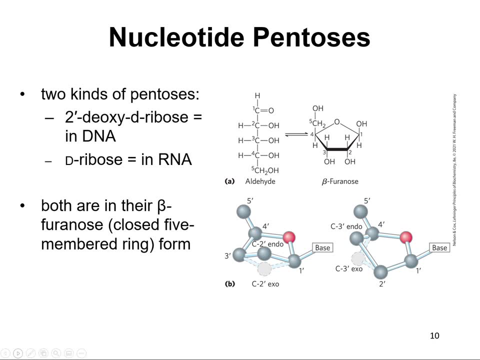 and uracil. so since they only exist in DNA or RNA, we don't have to worry about those distinctions. so there's two different kinds of pentoses, which we alluded to. they're both ribose, but we can either have deoxyde ribose, like in DNA- that's the, that's the D part- deoxy, or just plain old de ribose. 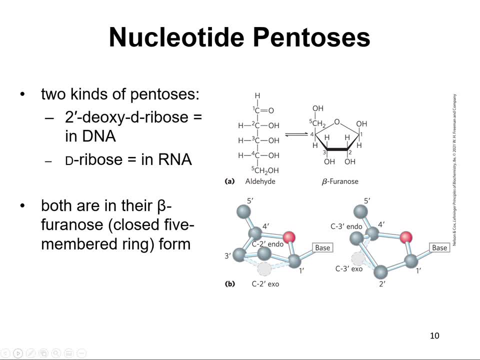 which is an RNA. they're both furinosis, closed five member ring. but again, the presence or absence of that hydroxyl group determines whether or not you're looking at a nucleotide that is for DNA or for RNA. this, as it's pictured, is for. 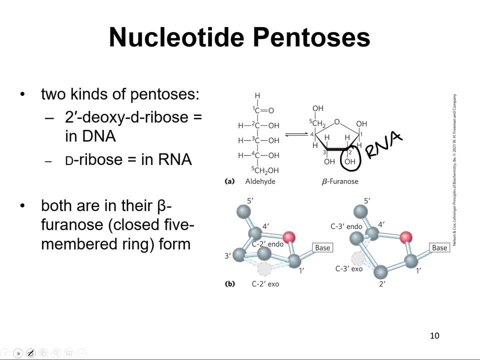 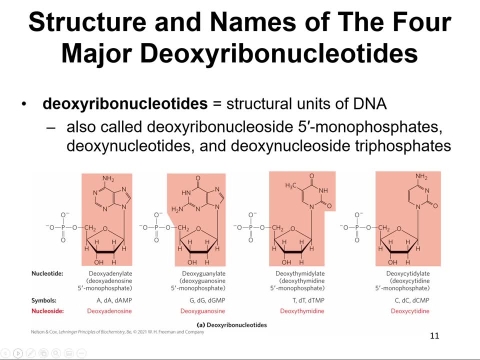 RNA deoxyribonucleotides- these are the structural units of DNA. there's lots of different terms that you can use, so I want you to be familiar with them all. it's kind of like learning the English language or any language where you have synonyms for things. this slide is going to be really helpful for recognizing the 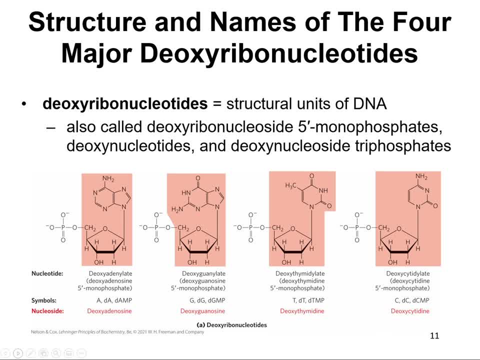 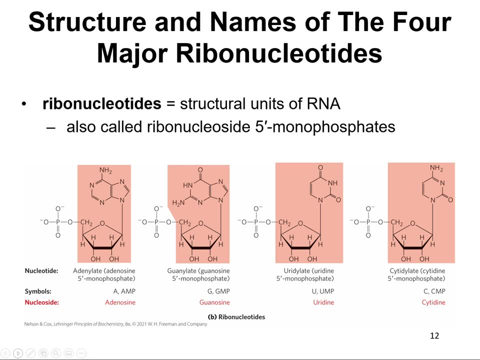 structure of a nucleotide and the structure of a nucleotide and the structure and getting to know the terminology for all of the deoxyribonucleotides, then we have the same thing for the ribonucleotides, and these are for RNA. notice that really the only difference is the presence of this hydroxyl group. 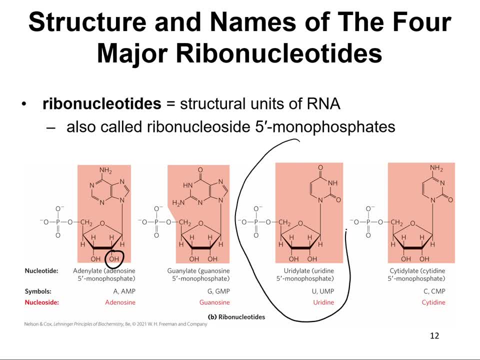 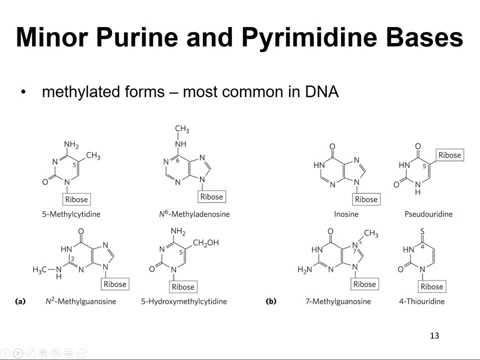 and also we're swapping uridine in for thymidine. they're going to be able to tell you that they they're getting. their DNA contains. these two subtypes of uridine and thymidine are similar. we're swapping uridine in for thymidine. there's also some minor peering in Purimidine basis. 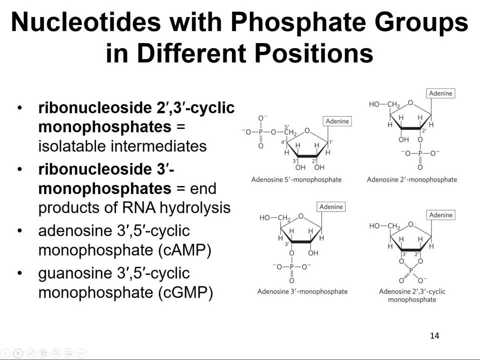 You can also have nucleotides with phosphate groups at different positions. You don't need to memorize the different positions, but, again, just be aware that this is a thing and they have a purpose. What you'll definitely see when it comes to signaling is cyclic AMP and cyclic GMP. 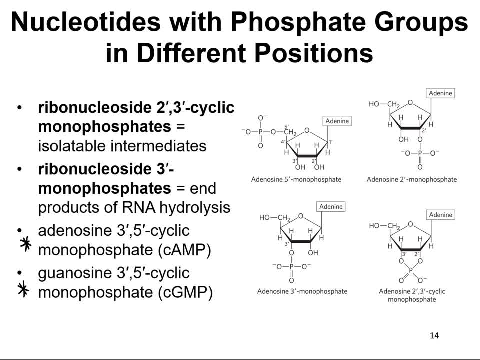 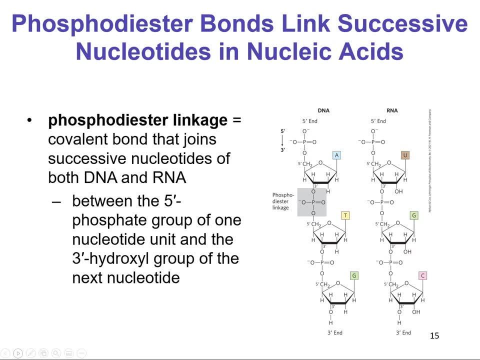 So those are definitely two important ones to take note of, Not because you need to know the structure, but just because it may crop up again in one of our case studies when we're looking at things that have to do with nucleotides. Now, we've got all of these building blocks, but we have to have a way of stringing them. 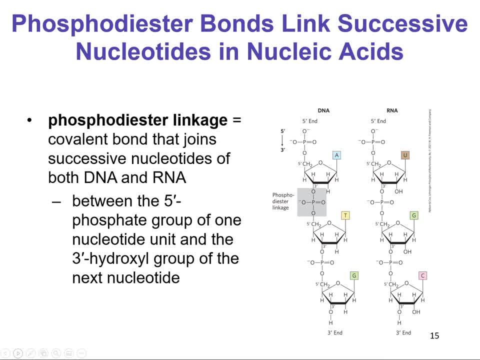 together. Otherwise we won't have a nucleic acid. The phosphodiester bond is what links all of the nucleotides in your DNA and your RNA. It's a covalent bond that joins all the nucleotides together. So what happens is you have a five prime end of DNA or RNA. 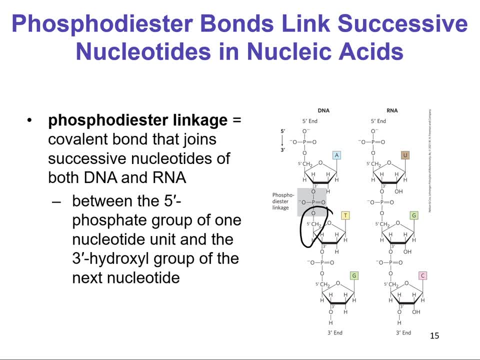 So we're looking at this area. It is going to link up with the phosphate of the three prime of the previous nucleotide. There's going to be a covalent bond made And I'm not going to require you to know the chemistry and draw the arrows for how the 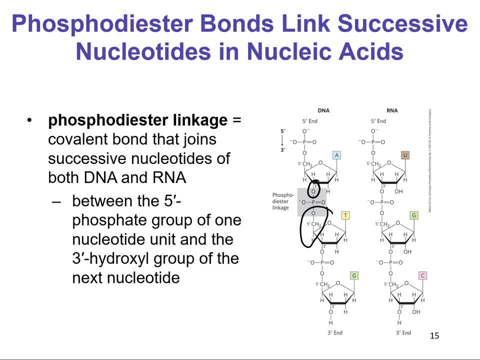 phosphodiester bond is formed. But just know that this is what it's called. It's a phosphodiester bond And it's between the five prime phosphate on one nucleotide and the three prime hydroxyl of the next one to be added. 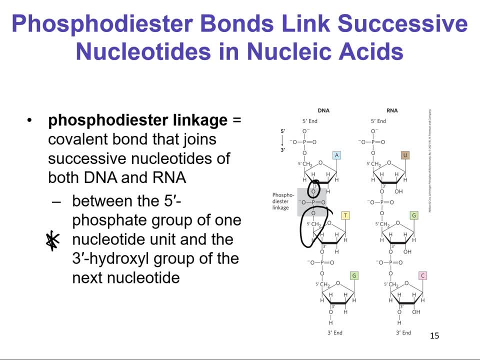 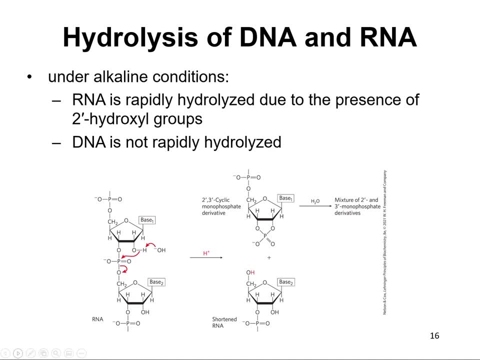 So you definitely want to know that DNA and RNA can actually be hydrolyzed under alkaline conditions. DNA is not as rapidly hydrolyzed, but RNA absolutely is, And the reason for this difference is because of this two prime hydroxyl. 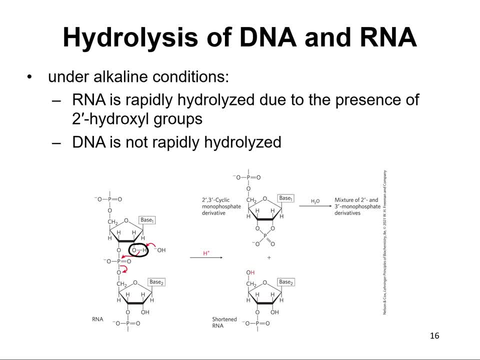 If you have a base that can steal away a hydrogen from that free hydroxyl group, then you're going to need a hydrogel. Then you suddenly have electrons that can do some work And just like- let me erase that because I'm completely covering that P in the phosphate. 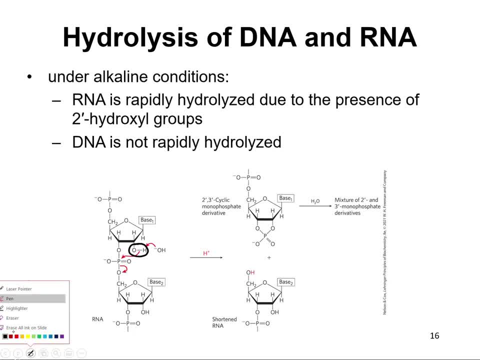 Whoops, Just having all types of issues here. Okay, Let's try that again. These electrons can attack that phosphate because it's got a partial positive charge, Just like a carbonyl carbon. Okay, It's got a partial positive charge. 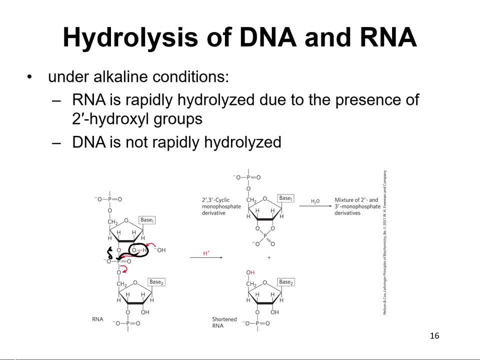 That phosphorus in that phosphate molecule has a partial positive charge, So it is ripe for chemistry when it comes to hydrolysis and you have a good nucleophile. So once you do that, then you can kind of break it apart. So you have, you know, either a break in an RNA strand or something like that. 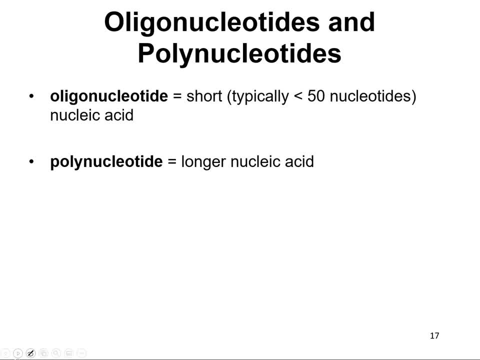 Okay, Okay, I'm going to go ahead and show you how to do that. There's some more terminology and you'll see a lot of uh similarities when it comes to talking about DNA and RNA, so nucleic acid structure and protein structure. 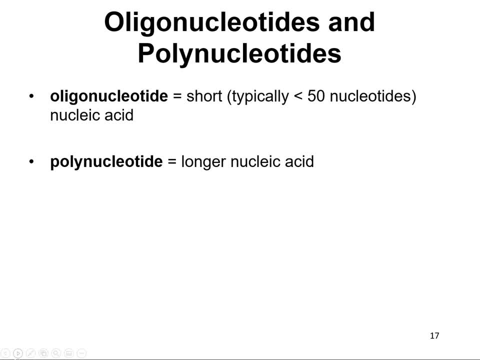 Be thinking about the similarities in terms of the terminology because, as we build up, we're eventually going to have a final, and that final is going to be taking all of these concepts and linking them together. I'll do my best to point out the areas that you should be looking at and trying to forge. 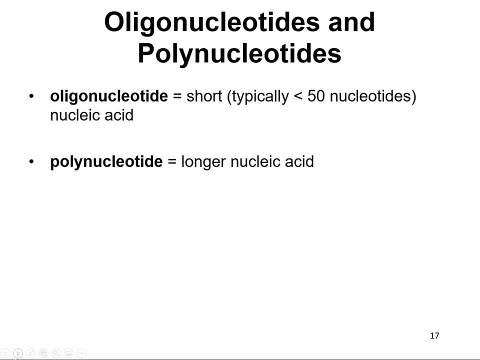 connections between but um, you'll need to do that on your own too. So come to me with questions about how to do that if you need help. but you can think about biochemistry, as you know, all of these different players. we've got all these different. 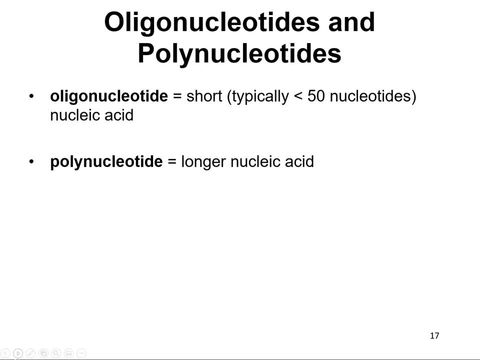 teams in the body. We've got team protein, team carbohydrate, team lipid, which we're going to be introduced to next week, And all of these things are coming together and they're just having all it's like a a free for all fun day. 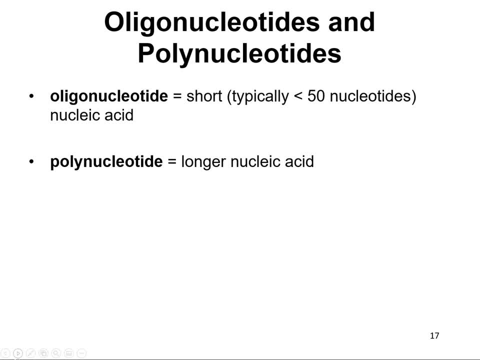 You got kickball, you got dodgeball, three legged races, all kinds of things, and they all have to interact with each other, But there's certain rules for how and when they interact. We're learning the terminology so that we can look more closely at those interactions. 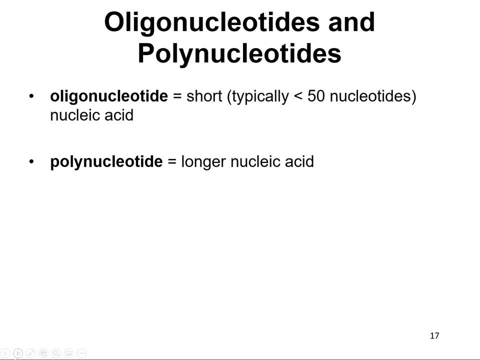 and how all those interactions together form a functional human being or other. you know species like some animal or something, Right, But we're focused on people. Let's just be honest: Medical field- We're focused on people here. So that was a brief aside to try to help bring together why we're looking at all of these. 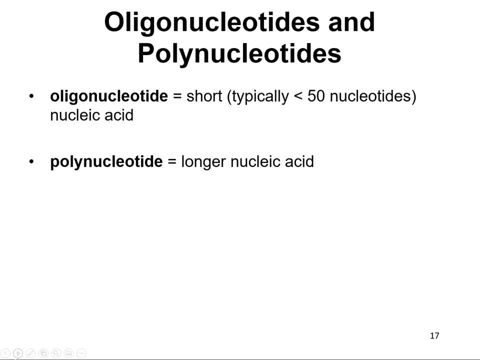 things. It's so easy to get stuck in the terms and all the things you have to memorize and forget the bigger, broader picture of learning the players, so you can see how they work together. All right, So, speaking of learning players, some more terminology. 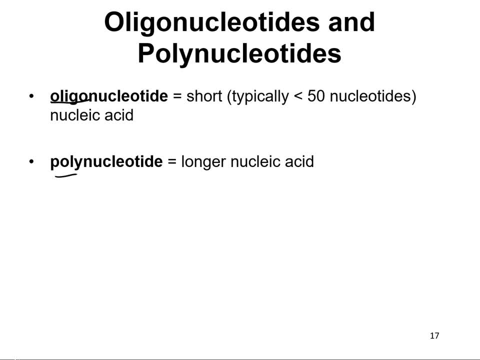 We've seen a ligo and poly several times now, so you probably already have an idea of what we're looking at here. An oligonucleotide is a short nucleic acid, So we're talking like less than 50 nucleotides. 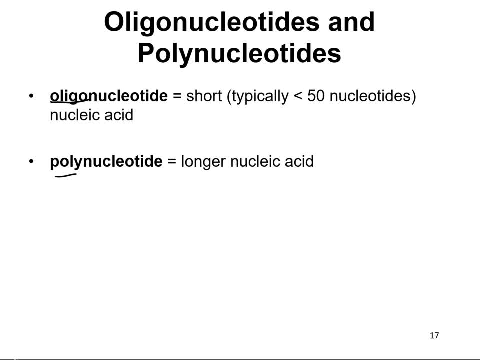 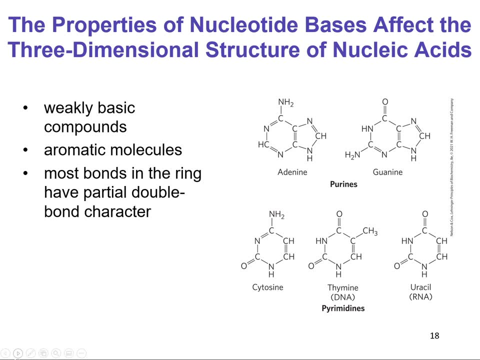 Polynucleotide, much longer nucleic acid. So the properties of the bases affect the three dimensional structure of nucleic acids. All of the bases are weakly basic compounds. They're aromatic, They're aphrodisiac. They're aphrodisiac. 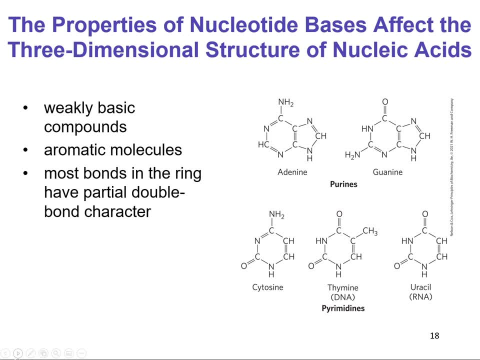 And most of the bonds in these rings have some partial double bond character, So that makes them pretty rigid and fairly planar. We're not going to talk about, you know, the small differences between the purines and pyrimidines in terms of. oh well, the purines, have you know, are planar. 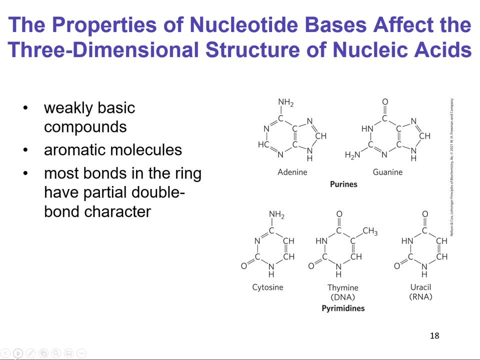 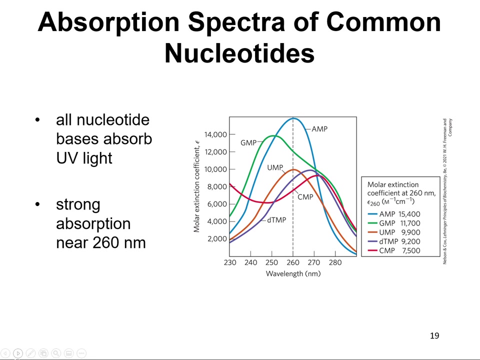 The pyrimidines. maybe they pucker a little bit. We're not talking about that, All right, All right, All right, familiar with these basic characteristics of being weakly basic, aromatic, aromatic and the double bond character: all nucleotides absorb UV. 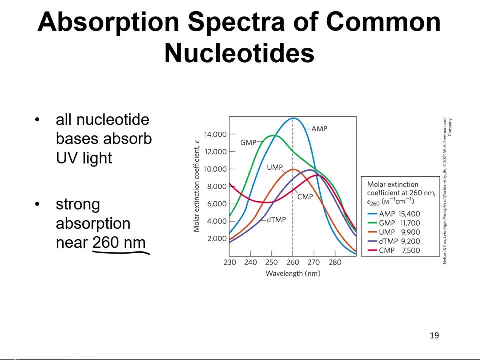 light and they have pretty strong absorption- around 260 nanometers- and this is key. in the lab, this is actually used to calculate concentrations of nucleic acids in solution. there are instruments called- well, I know that the proprietary name for the one that I'm thinking of is a nano drop, but there are. 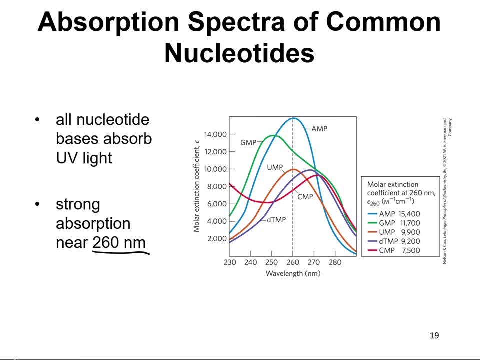 these little machines that literally fit on a table or a desk next to a computer, that you can put one or two microliters of your nucleic acid solution on and put the little lid down and it will. you can look at the absorption and it will. 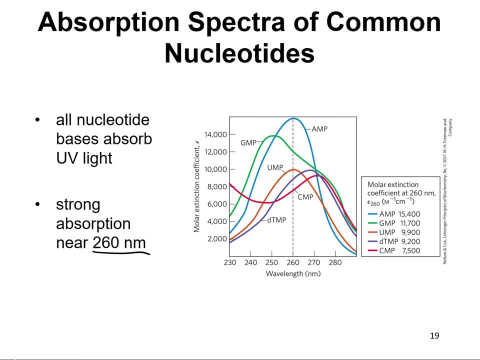 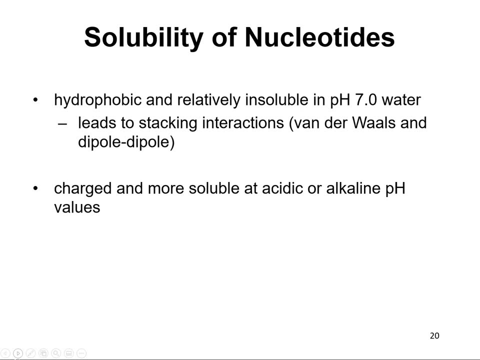 calculate the concentration of the solution based on its 260 nanometer absorbance and the molar extinction coefficient. if we're looking at nucleotides, they're actually pretty hydrophobic and so they're not really that soluble in water at pH 7. but if you have more acidic or 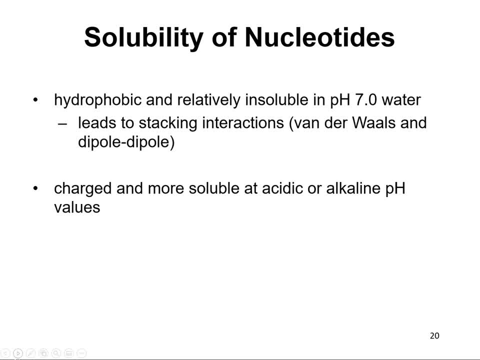 more alkaline conditions, then it's a little bit more soluble. but these things definitely don't want to be interacting with water at pH 7, and that's what we have a lot of in us, and we're around pH 7. so what do we do? well, 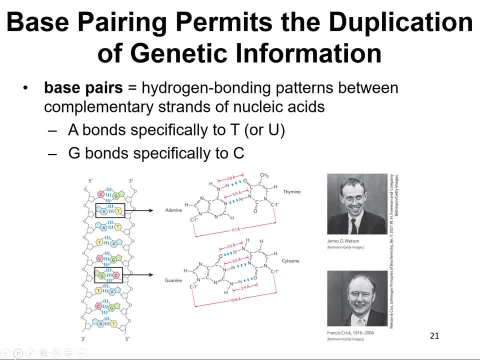 there's lots of stacking and base pairing. base pairing fulfills the requirement of keeping all of the hydrophobic stuff together and sequestered away while keeping all of the hydrophilic stuff on the outside. so why is that so? Watson and Crick- I'm sure you've heard those names. 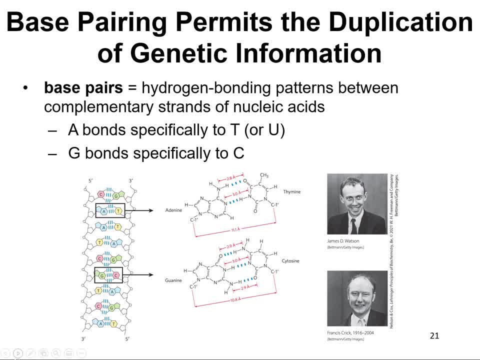 several times in biology And they are really instrumental in identifying the 3D structure of DNA. Base pairing is just the hydrogen bonding pattern between the complementary strands of nucleic acids, So typically you've got A bonding to T and DNA. It can also bind to U if we're talking about RNA. 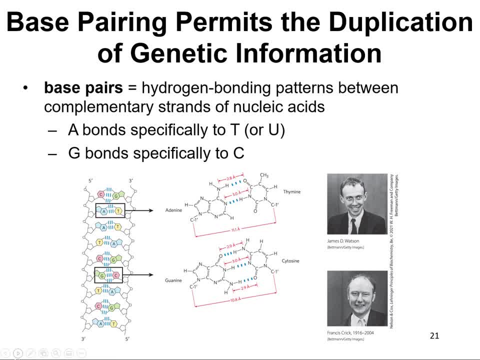 And then G and C pair together as well. What you can see in this blowout here is the interactions between A and T and G and C. When I talk about you knowing the structure of the bases and being able to draw it, I also 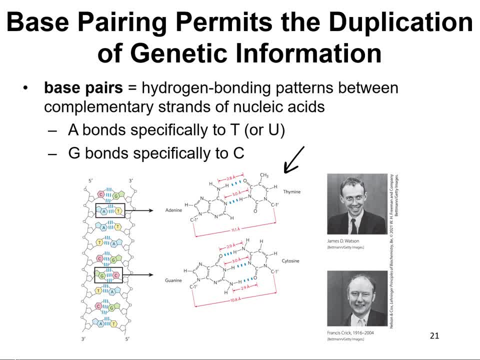 want you to know the structure of the bases. So typically you've got A bonding to T and DNA. You want to know where the hydrogen bonding happens. So we're going to talk about that specifically on a separate slide, But I'm just pointing it out now that that's something. 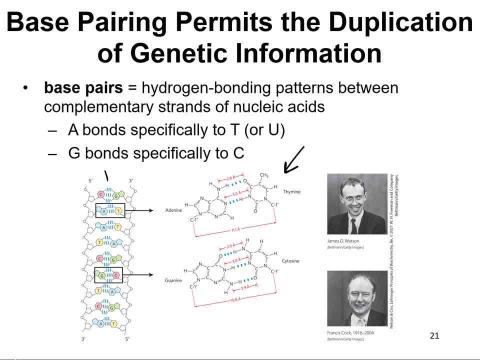 you'll need to know as well. But notice how we've got all of this hydrophobic stuff in the center And then what you have on the outside. so this part is your sugar phosphorous. This is your phosphate backbone. We talked about sugars in Chapter 7.. 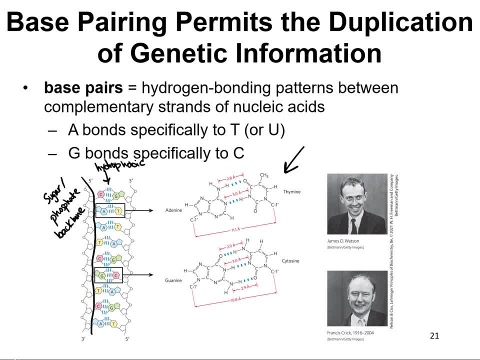 They need water to be soluble because they have all those hydroxyl groups that need some hydrogen bonding to keep them happy. And then we've got phosphate groups- this long phosphodiester chain- highly, highly negative. So those are right-field. 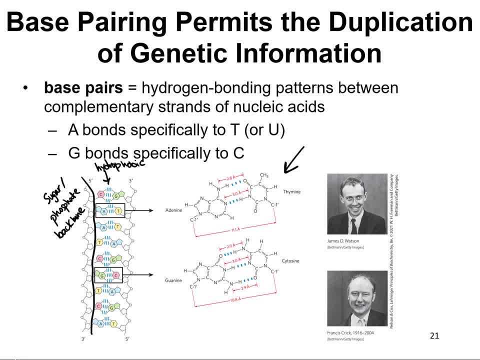 And then the second one is the hydrophobic group for hydrogen bonding. So it's just like a protein when you think about the 3D structure and the idea of sequestering away the hydrophobic region, AKA the nucleotides, away from. 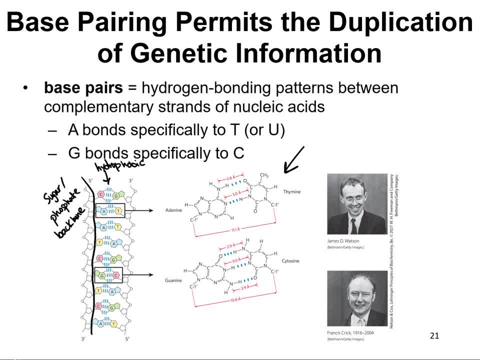 So I guess we'll call these the bases right, Because the whole thing is nucleotide. So the bases, the purines, the pyrimidines, they're facing each other and doing some hydrogen bonding, Which is another way of saying van der Waals. 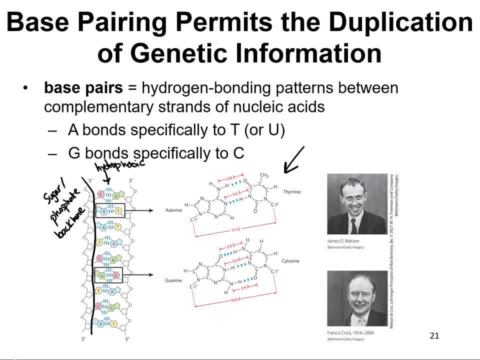 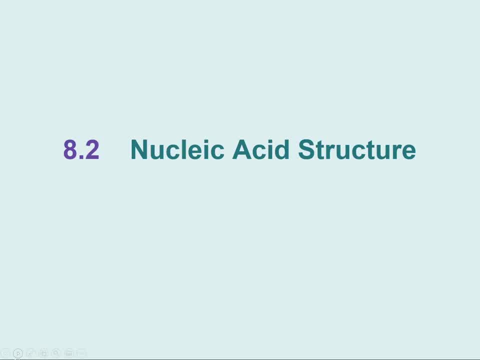 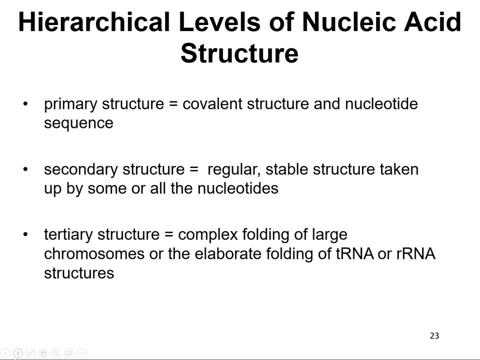 And then you've got the sugar phosphate backbone. that is incredibly hydrophilic and needs water to stabilize it. So now we're going to talk about nucleic acid structure in more detail. I was already getting to that, because I'm getting so excited. 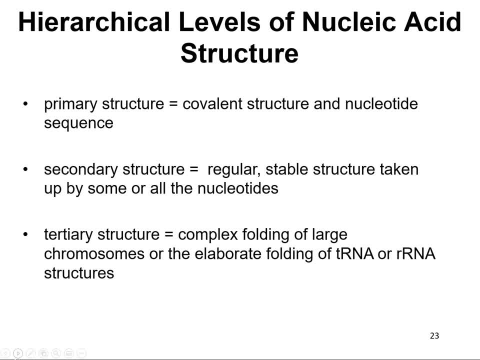 Nucleic acids is another big interest of mine. Just like with proteins, nucleic acids, nucleic acids have hierarchical levels of structure. We've got primary structure, And that includes the nucleotide sequence and the covalent structure. right. 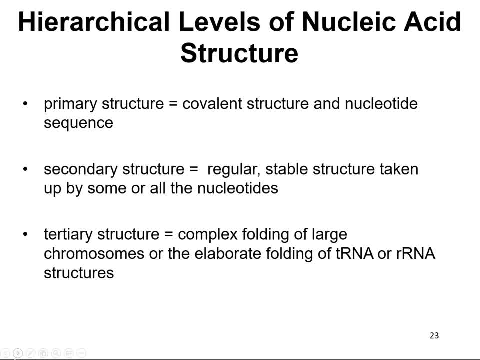 Then we've got secondary structure, which is regular, stable structure that's taken up by pretty much all nucleotides. okay. Then the tertiary structure. we're talking about the folding of large things. So we have large things like chromosomes or tRNA, rRNA. 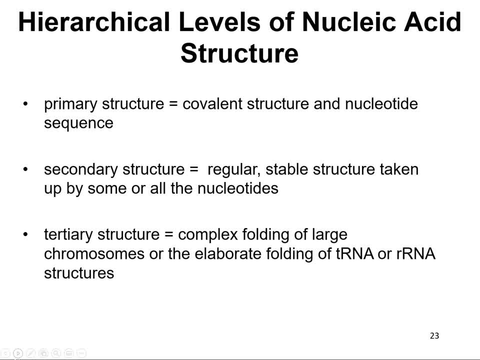 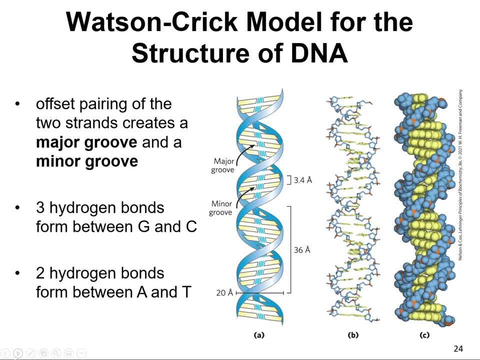 Those things have, you know, lots of different structural features in them. This is the Watson-Crick model for the structure of DNA. When you have two strands coming together, wound around each other, you actually create what's called a major groove and a minor groove. 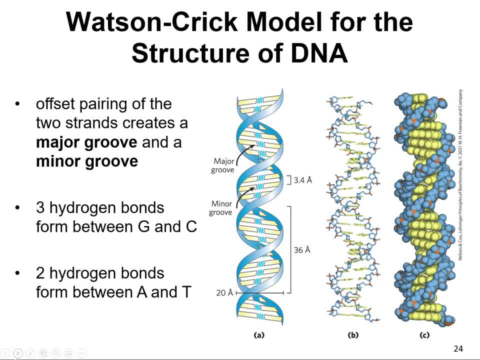 And these grooves are really important when it comes to protein binding and enzyme binding because they are specific, for you know, some bind major grooves, some bind minor grooves. So this is actually an important distinction. When you look at the ball and stick model here in the center, 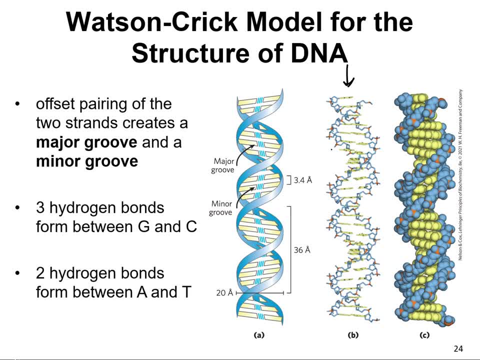 I think that the major and minor grooves are much more visible. So we've got a major groove here, That's this space here. That is much, much bigger than our minor groove, which is here. I remember being in grad school and having to look. 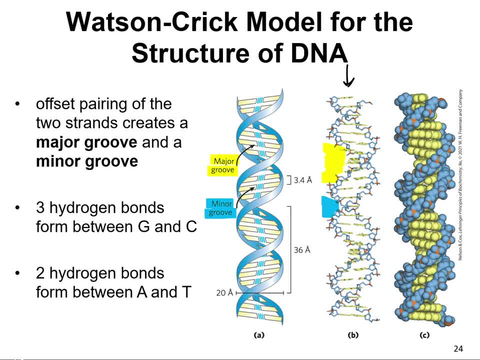 at a structure and identify major and minor grooves, and it was such a pain. It was one of those things that took me a little bit to really understand And it was just so frustrating to be like, okay, I'm supposed to just look at this structure. 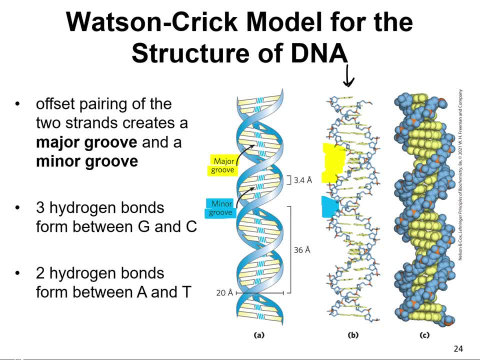 and know what a major groove is and a minor groove is just based on this. Oh my gosh. It was one of those like I'm ready to tear my hair out and eat it type of moments, But I got there. 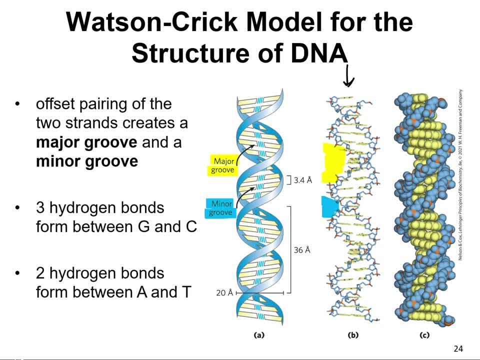 I finally got it. Anyway, in addition to the major grooves and the minor grooves that we create, we also have to talk more specifically about the hydrogen bonding between G and C and A and T. Between G and C, you're gonna have three hydrogen bonds. 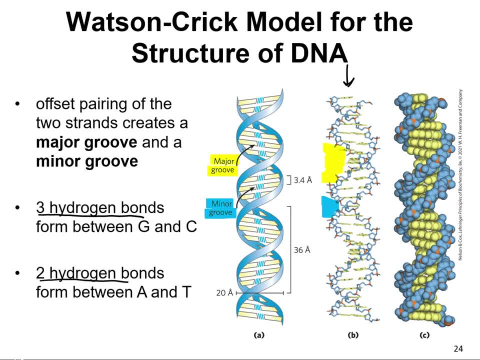 Between A and T, there's gonna be two. This is the kind of traditional bonding. okay, There's also something in your book that talks about Hoogstein pairing. We're not talking about Hoogstein, okay, Hoogstein is another one of those things. 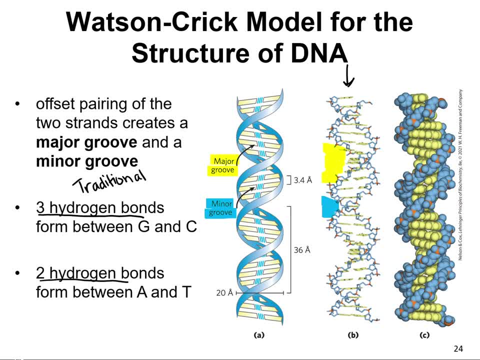 that plagued me initially when I was in grad school, But I finally understand it. But Hoogstein-base pairing- it absolutely is relevant and it's something that needs to be considered if you're interested in DNA and RNA and the proteins and enzymes that bind them. 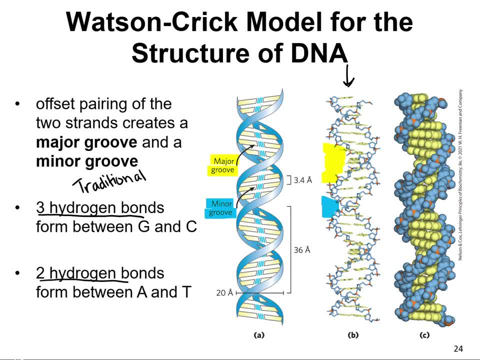 and do chemistry with them. However, for our purposes, I'm not going to make you understand Hoogstein pairing, But it's just an alternate way of the bases interacting. so it's different hydrogen bonding that causes for differences in structure that can be recognized by different proteins. okay, 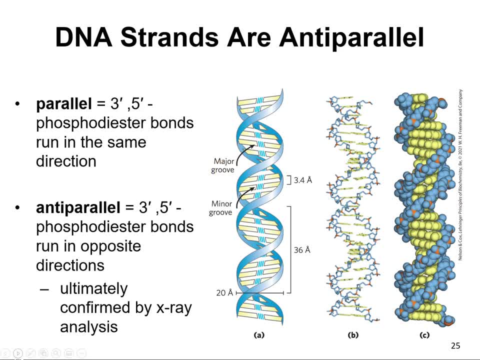 So there's that- More descriptions about DNA. The strands of DNA are anti-parallel, So there's two strands. right, It's a double helix. I can't believe. that's the first time that I'm saying that. I think it's one of those things that everybody knows, that right. 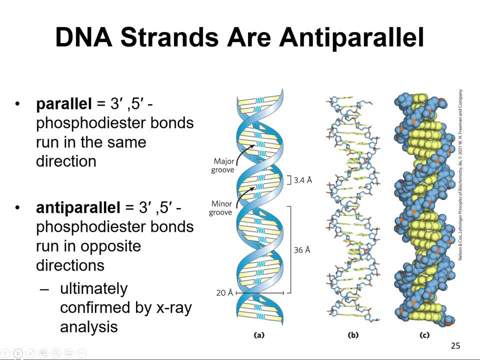 It's a double helix. Anyway, that should be stated. DNA is a double helix And the strands are anti-parallel. So what that means is we've got these two different strands, So I'll kind of color. There's one strand. 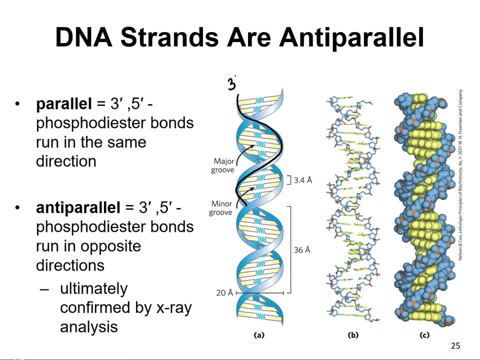 I'm not going to color the whole thing And we'll say this is the three prime end, And we get all the way down here. This is the five prime end, The second strand, all the way down here the five prime is actually up top with the three prime of the other. 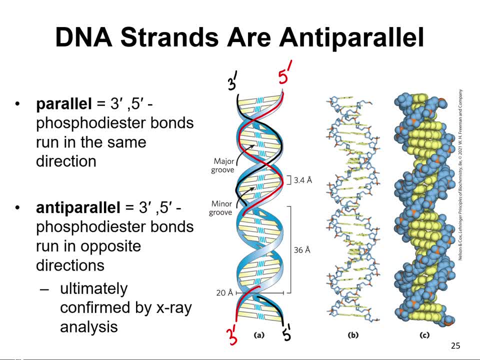 So these are anti-parallel. The phosphodiester bonds are running in opposite directions. It's going to be really important to understand that when we're looking at DNA and RNA metabolism, because understanding the anti-parallel nature of double-stranded nucleic acids 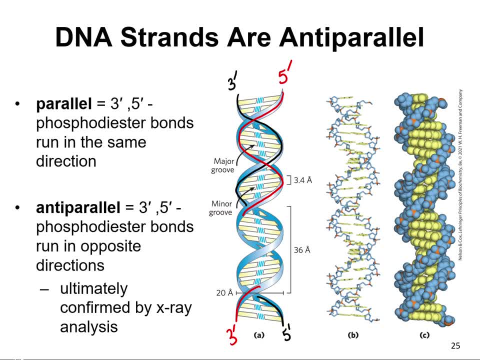 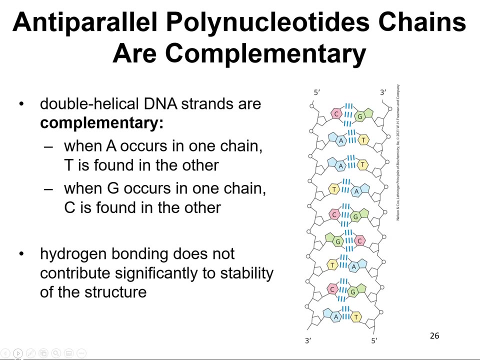 will help you understand the mechanism for how we replicate and repair these molecules. So it goes without saying that parallel means you would have three prime and five prime running in the same direction. The anti-parallel chains are complementary, So that's how we get our base pairing. 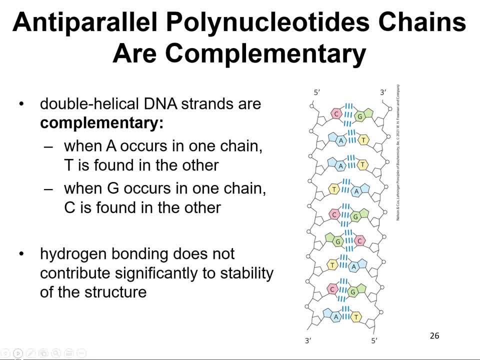 If you see an A in one train, you're going to find a T in the other, G in one, C in the other. Surprisingly, the hydrogen bonding between the bases doesn't contribute significantly to the stability of the DNA. I know. 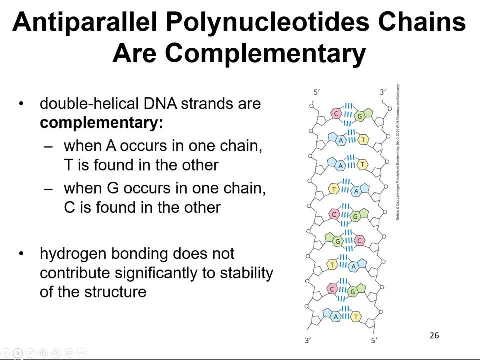 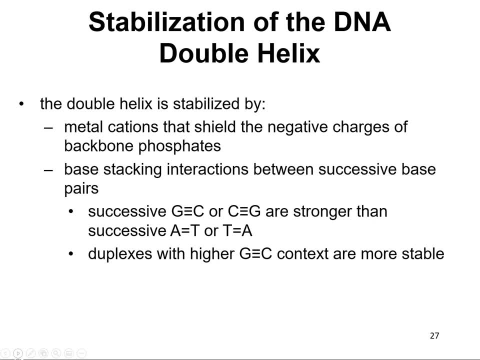 I know Mind-blowing, It doesn't contribute to it. Then what does? What actually helps the most is there's a ton of metal, a ton of metal that is protecting the negative charge of that phosphate backbone. So the outside. 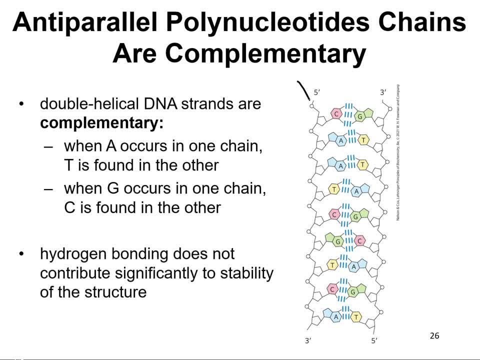 I'm going to go back just for a second here. So this part, the circles and the pentoses. this is known as the phosphate backbone. You may also see it called the phosphate sugar backbone. They all mean the same thing. We're talking about the phosphates and the pentoses. 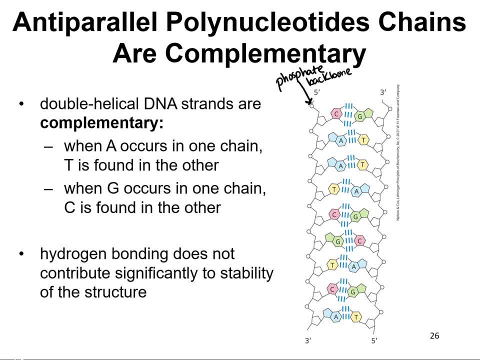 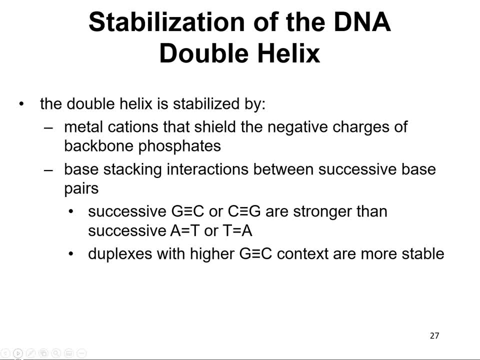 of all of the different nucleotides, and that's on the outside of the double helix. All that negative charge from the phosphates has to be covered, okay, And you cover that with metal When you're dealing with DNA or RNA. 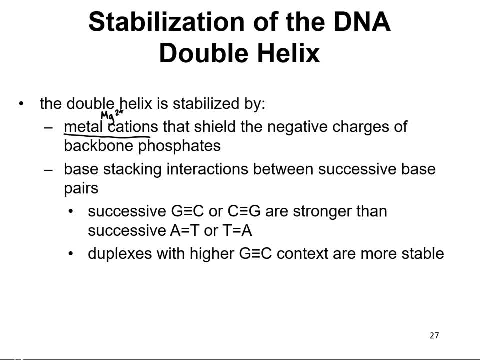 you're typically going to see a lot of magnesium ions, So that's Mg2+, And those ions will interact with the backbone to shield all of that negative charge. That helps to stabilize the structure of DNA. The other thing that helps with stabilizing the structure: 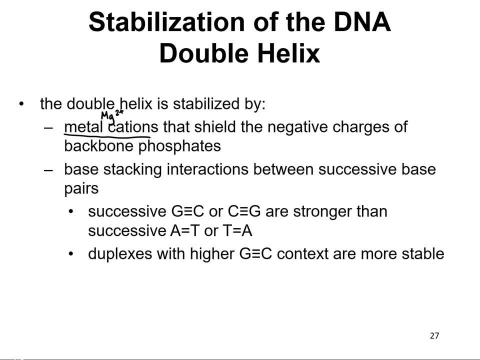 still has to do with the nucleotides, but it's not the hydrogen bonding between them, It's base stacking interactions. So when you stack the base pairs, there's van der Waals happening between each layer. So if we were to represent all of the pairs, 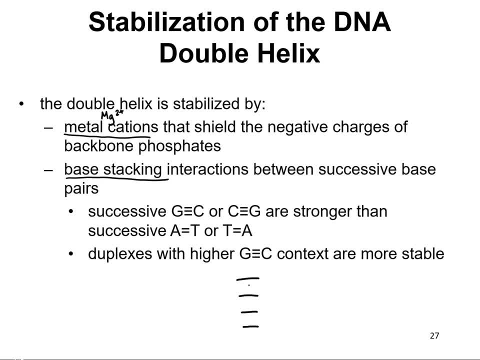 the base pairs like that. they're stacking in between. So this is the van der Waals, Which is also known as base stacking. here. Interactions- Base stacking interactions- are specific to nucleic acids. It falls under van der Waals. 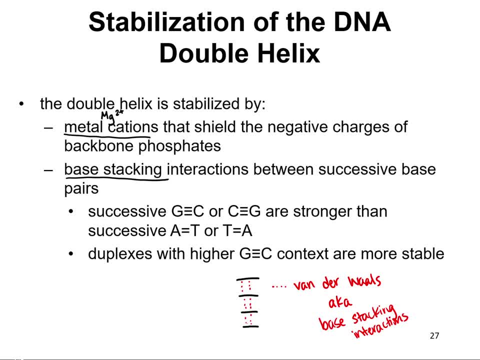 Just to try to help you keep all the terminology straight. All of those stacking interactions stabilize the double helix of the DNA. If you have more GC compounds, then you have a more stable molecule, And this comes into play if you're doing work with nucleic acids. 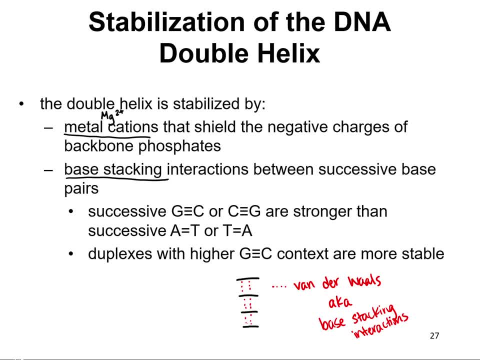 Often times you will need to purchase or make different oligonucleotides for cloning and all kinds of purposes, And if you have a lot of GC pairs it can actually be a little bit harder to work with. But if you have a lot of GC pairs, 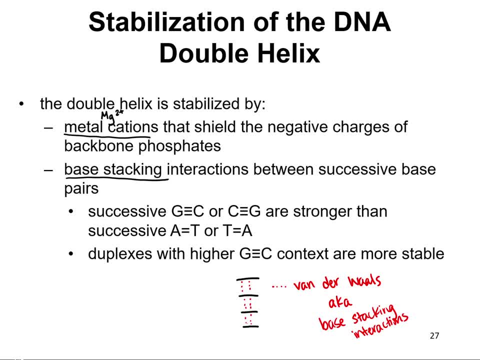 it can actually be a little bit harder to work with, Because it's super stable and sometimes they actually form different structures that you don't really want. So it's something that you have to keep in mind experimentally when you're trying to make or purchase oligonucleotides. 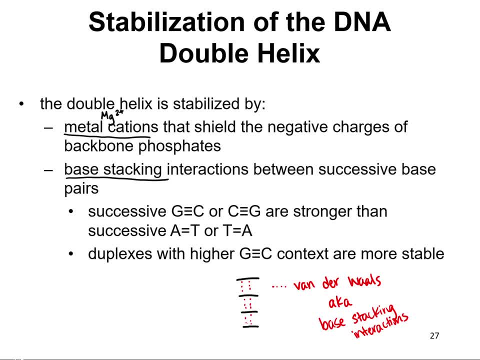 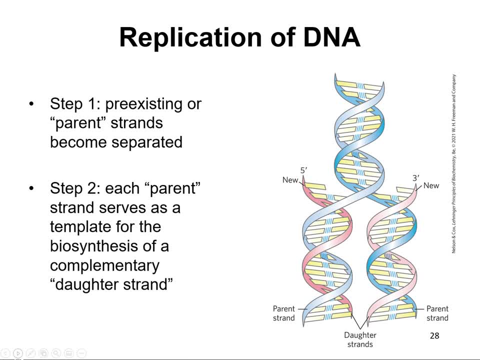 That's completely an aside. If you're interested in that kind of thing, we can talk about it all day long. So we already know that DNA has to be replicated. These are just the very, very few. These are just the very very few. 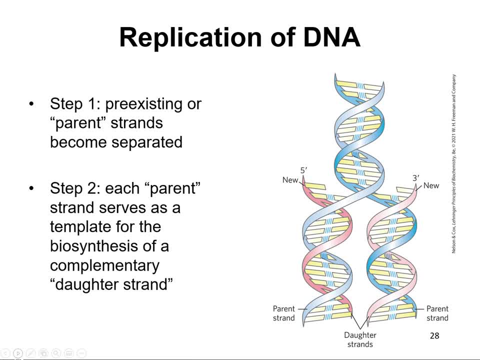 basic steps of DNA replication. Again, we're going to get into that when we look at DNA and RNA metabolism towards the end of the course. But the first step in replication of DNA is you have to separate the parent strands. So in its current state it's very stable. 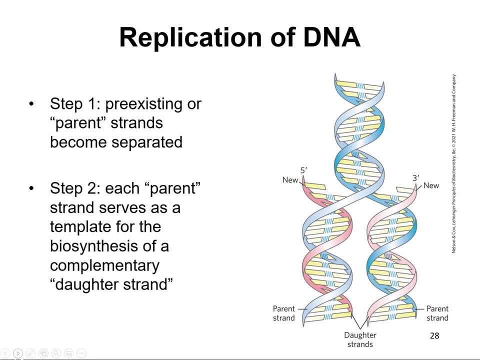 The information is not accessible. You separate those strands and each of them serves as a template for creating two new daughter strands. So each new molecule of DNA has one parent strand and one daughter strand. The daughter strand is the one that is newly synthesized, that's complementary to the parent. 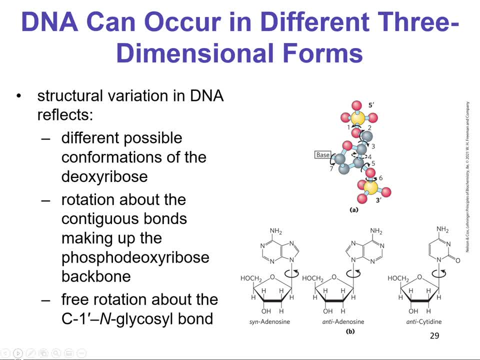 DNA can occur in three in different 3D forms. So those structural variations reflect the different conformations of that deoxyribose. So remember that sugar. there are some areas where it can turn, The bonds are free to rotate, And then there's also rotation. 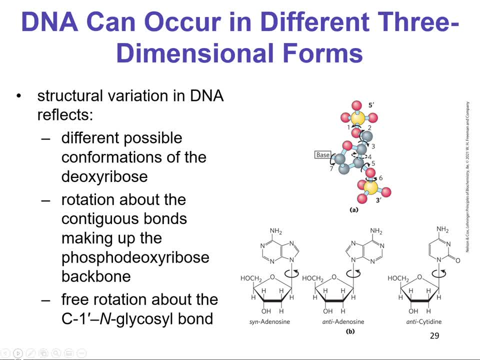 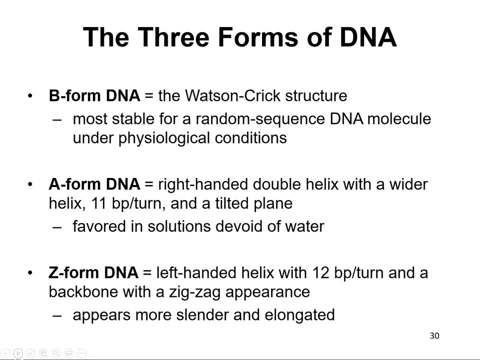 in terms of the about the phosphate backbone, the phosphate-sugar backbone, The three forms of DNA, we've got the B form, which is the most stable. That's the Watson-Crick structure. It's what you see everywhere And that is relevant for us, because 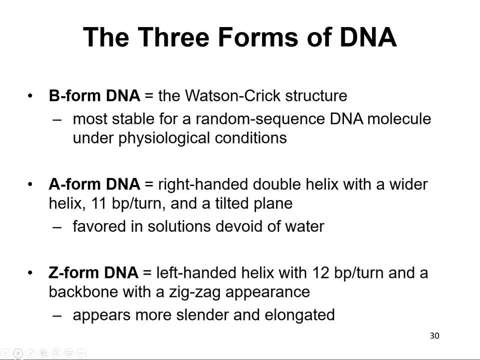 you know, that's what you see under physiological conditions. You can also get the A form of DNA and that's a right-handed double helix that has a wider turn, And I'll show you some pictures of this in just a second. 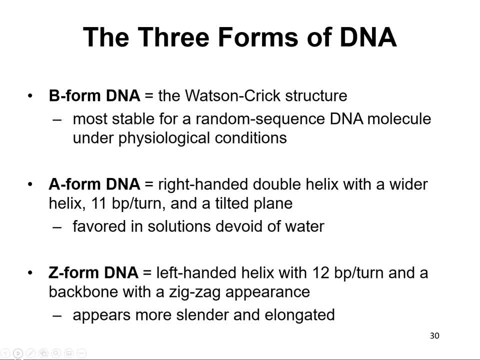 You don't need to know how many base pairs per turn, but you should know the difference between B form and A form, And A form is favored in solutions that don't have water, So think about organic solvents and things like that. Then there's the Z form. 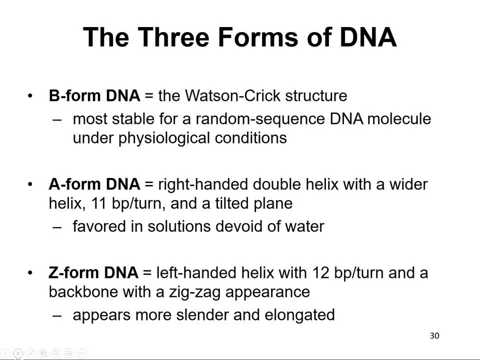 which is totally you know. just it's doing its own thing. It's a left-handed helix and it's, you know, got a zig-zaggy appearance and it's kind of elongated and slender in comparison to the other forms. 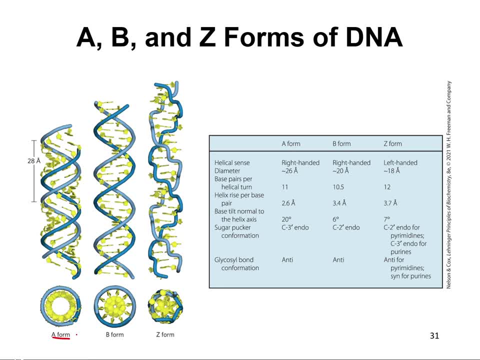 So here we go: A form, B form, Z form. You've got a table on the right-hand side. You don't need to know all the numbers like the diameter of the molecule and how many base pairs per turn and stuff like that. 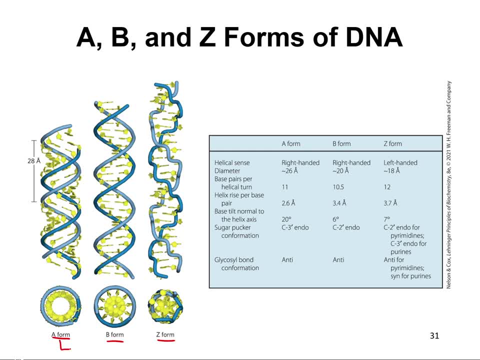 But you will need to be able to compare A form, B form and Z form in terms of you know, right-handed versus left-handed And A form. you're going to see that more so in you know organic solvents. 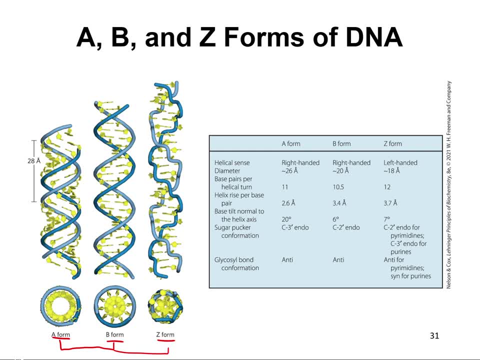 You're not going to see it really in water. B form is physiological. It's the Watson-Crick structure. Z form: just know that it's left-handed and it's got kind of a zig-zaggy appearance with that phosphate-sugar backbone. 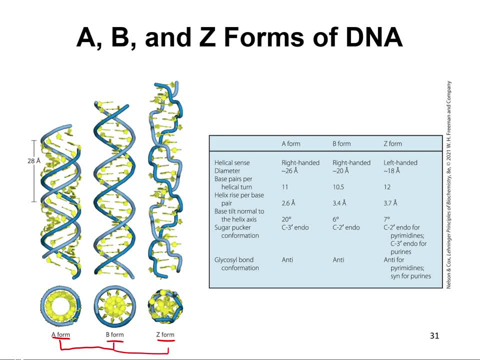 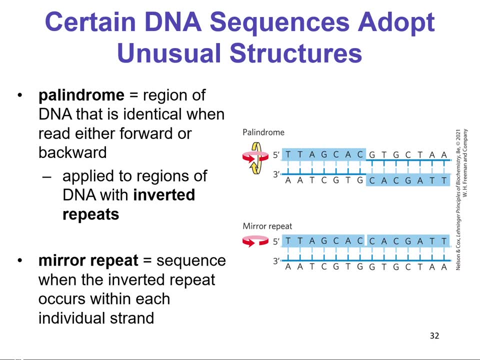 and it's more slender. There's some DNA sequences that adopt some strange structures, One particular region. we're looking at palindromes, So a palindrome is something that is the same whether it's read forward or backward. We have words that are like that. 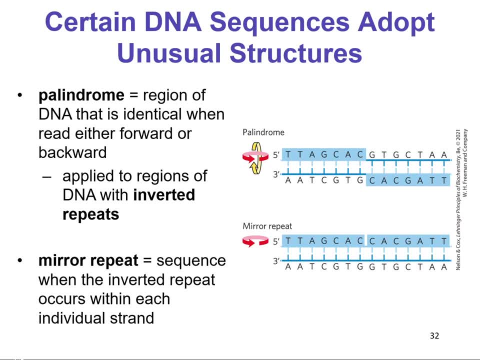 It's the same thing in DNA And in DNA, what we've come up with experimentally is- and some of these are just found in nature, in bacteria for sure. is these things called restriction enzymes or restriction? We perform restriction digests. 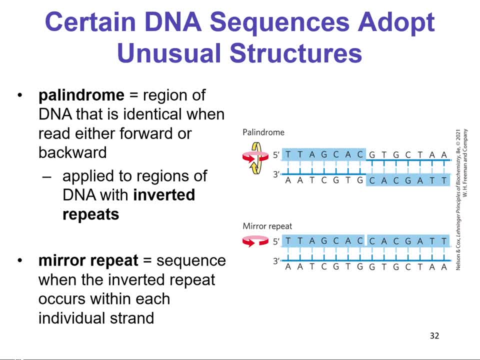 That means chewing up specific pieces of DNA or RNA or making a cut. okay, They usually recognize palindromes, So you'll get an enzyme binding here and you'll also get an enzyme binding here. But these particular places are where you can see. 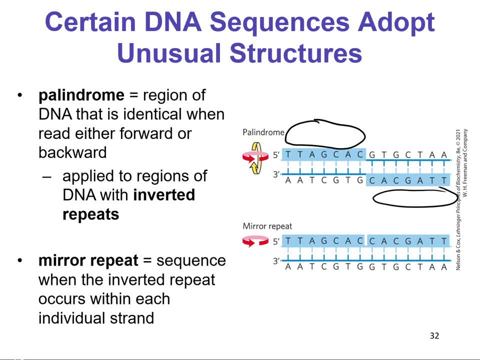 some different structures in the DNA, You can also see a mirror repeat. So that's when you have a sequence and then that sequence is like inverted and repeated. So if you had a mirror right here then you would see that mirror repeat. 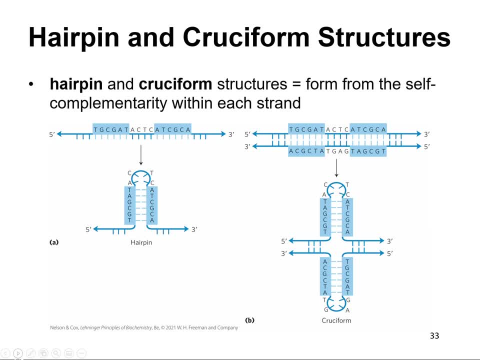 Some of the structures that you can see. We'll talk about hairpins and cruciforms. So a hairpin can form when you've got two complementary pieces of nucleic acid that are separated by a short stretch. They can see each other and say: 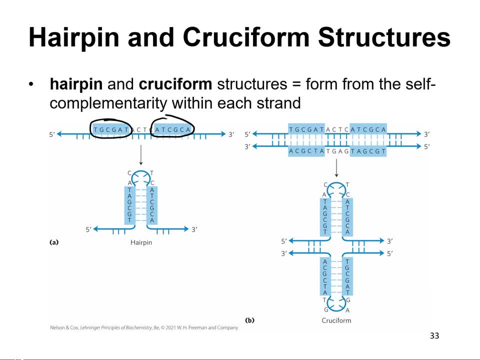 oh hey, we can base pair. So you get this little circular piece at the top where there's no base pairing, But then you have this complementary section here that's holding it together. That's a hairpin And it kind of looks like a bobby pin. 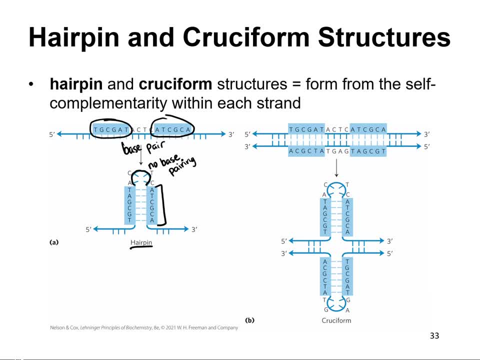 The next form that you can have is a cruciform, And that's essentially like a hairpin gone crazy. So we've got two hairpins that come together because we've got all this complementarity, So we've got a double helix, right. 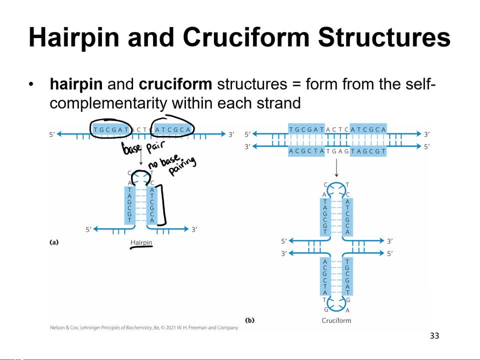 that's already got its own base pairing going on. And when you've got these two regions of complementarity so close to each other and then you've got just kind of normal sequence here, then it's going to end up forming a cruciform. 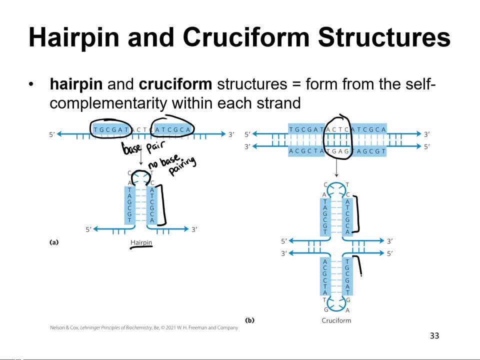 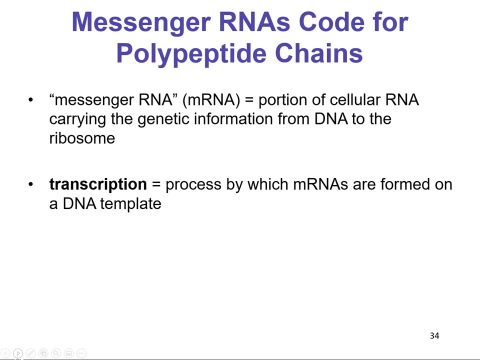 where you have these two regions of complementarity having some base pairing and then you've got no base pairing going on at the top. Let's talk more about RNA, because RNA is really where you see a lot of these crazy structures: mRNA, the messenger, RNA. 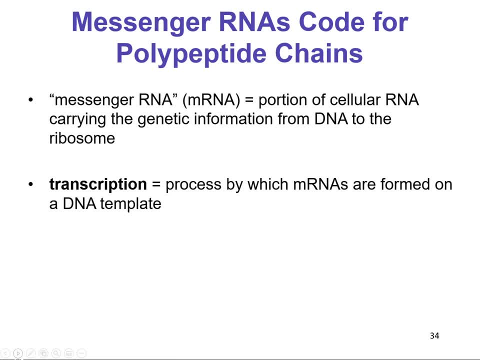 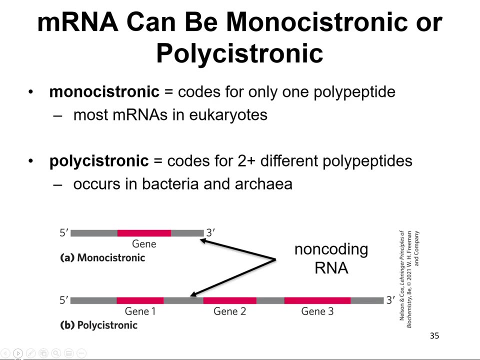 that is what helps to carry the genetic information from DNA to the ribosome Transcription is what that process is called, and we'll talk about that later on in the course, When you form DNA or when you form mRNA. excuse me, 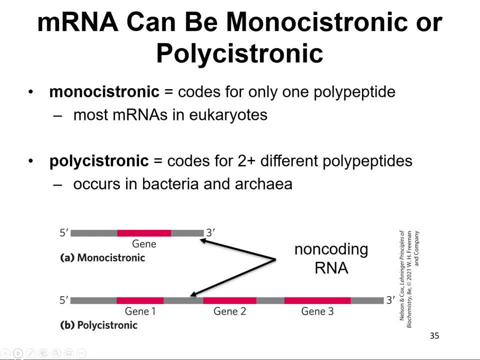 you can have monocystronic or polycystronic. Monocystronic means that the mRNA codes for one polypeptide, So one mRNA equals one polypeptide. But you can also see polycystronic, and that means that you've got one mRNA. 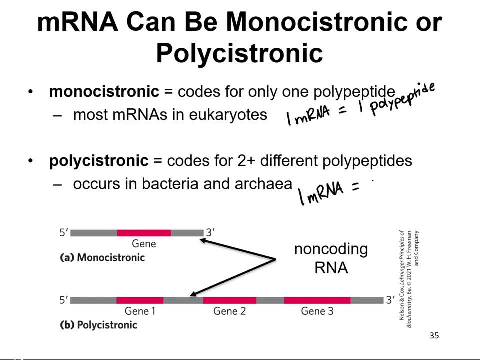 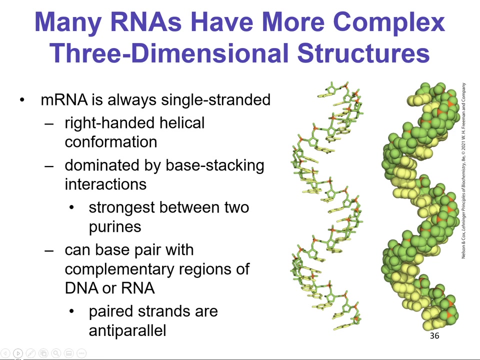 that leads to two or more different polypeptides. You see that a lot in bacteria, where you have one super long mRNA transcript and then you actually end up making like 10 proteins. mRNA is always single-stranded. It's got some other business to do with the ribosome. 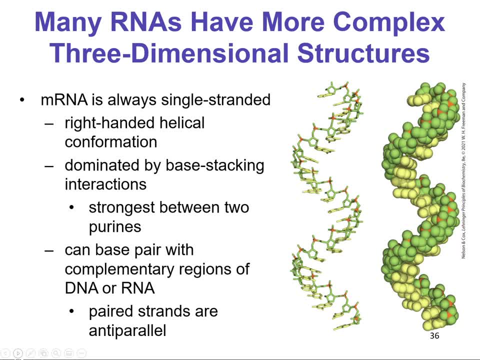 and it needs to be available to interact with the ribosome and those tRNAs that are bringing in the amino acids. So it doesn't have time for another strand. It's got enough relationships. It doesn't need the relationship of another RNA strand too. 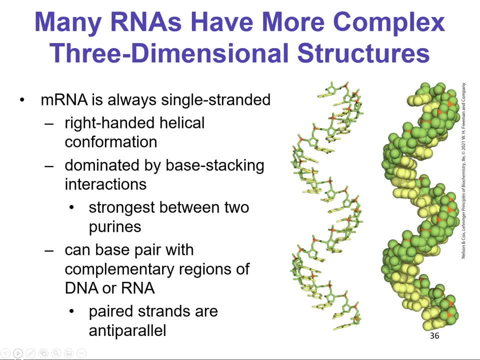 It forms its own right-handed helix And the base stacking interactions are what stabilize this structure. It's strongest between two purines, So remember the purines are the ones that have the double ring structure. So when you have long stretches of purines, 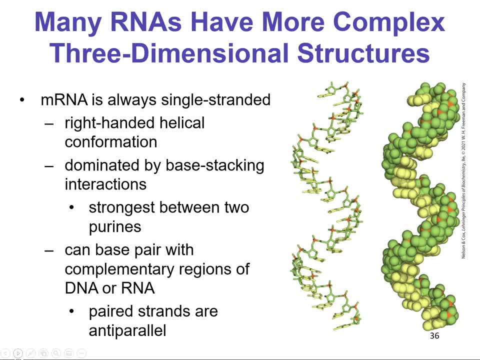 that helps with the stability of the molecule. mRNA can base pair with complementary regions of DNA or RNA. mRNA can base pair with complementary regions of DNA or RNA. mRNA can base pair with complementary regions of DNA or RNA. And when it does that, 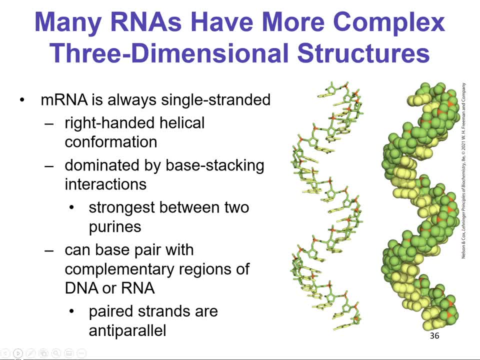 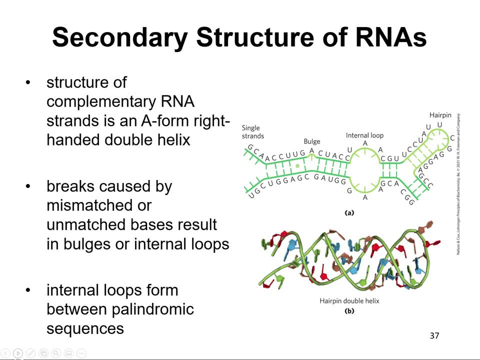 it is anti-parallel, just like with DNA, the two DNA strands, Secondary structure of RNA can get pretty wild. The structure of two strands of RNA that are complementary is actually the A-form, So DNA. B-form RNA, So DNA- B-form RNA. 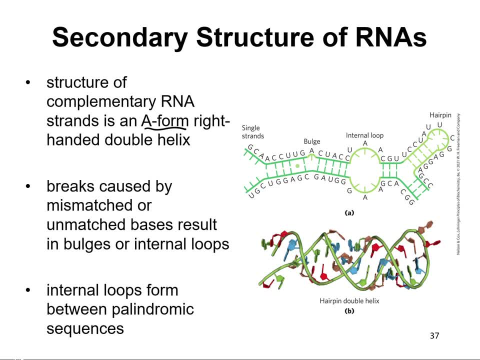 So DNA B-form, RNA A-form, A-form- Right-handed double helix- Right-handed double helix. There can be breaks in the structure that are caused by mismatches or unmatched bases And that can result in bulges and loops. 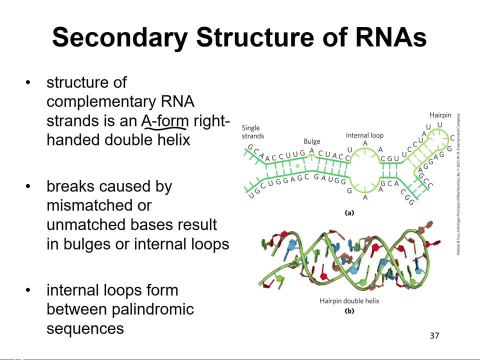 and all kinds of things. You've got internal loops between palindromic sequences. You've got internal loops between palindromic sequences, So you don't have to necessarily know all of these things on the slide, Just know that. secondary structure of RNA. 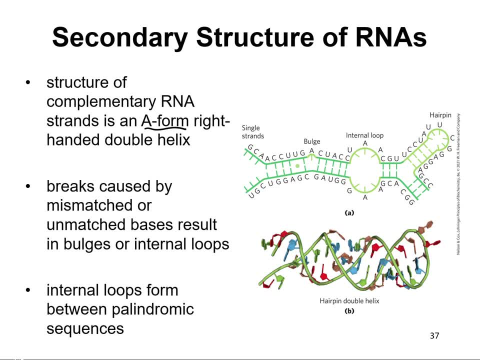 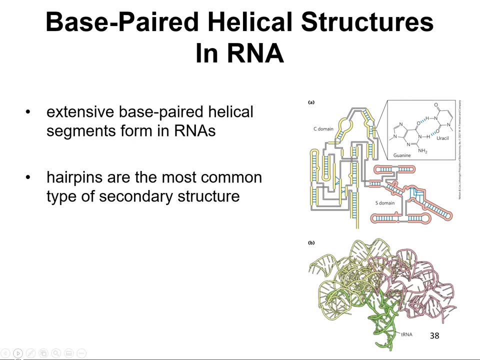 structure of RNA can be pretty wild. There's a lot more going on than with DNA. DNA, you've got your double helix B form. that's it All day, every day. RNA- much more complex. You can have some base pairing in helical sections in RNAs, especially like tRNA or 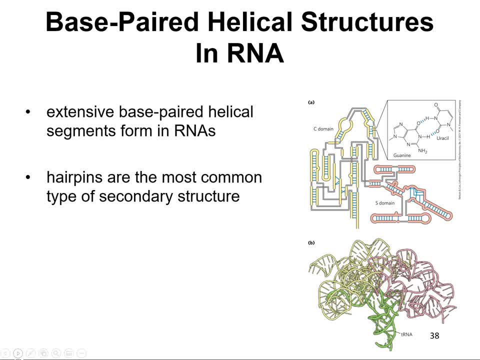 non-coding RNA. So what's shown here is a tRNA. This is a topology diagram, Just like with proteins, it shows the secondary structure And these tRNAs are pretty huge, So they have different domains: the C domain, the S domain. You don't need to know anything about tRNA. 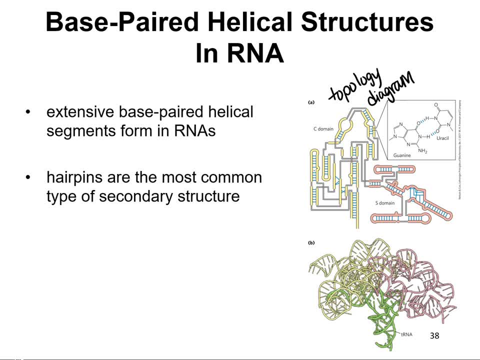 specifically, but there are specific domains. within the tRNA There's a place where the amino acid binds, So there's chemistry there that allows for the attaching of that amino acid to the tRNA. Hairpins are really, really common. It's the. 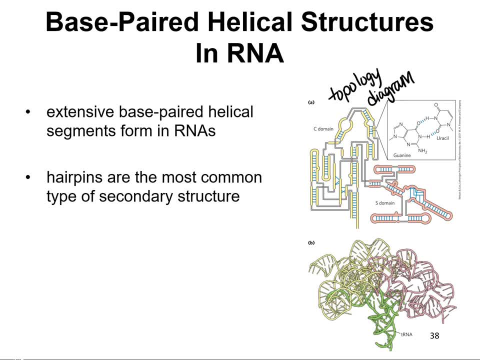 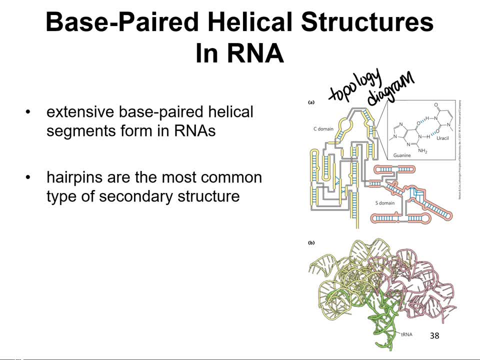 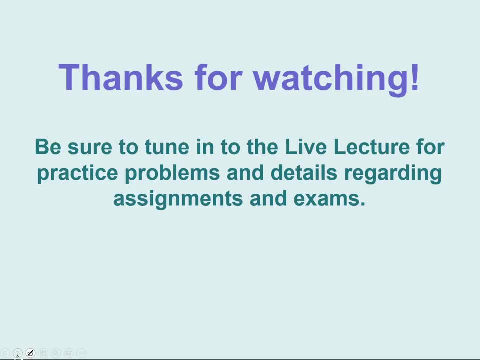 folding. I think it's beautiful. tRNAs are very hard to find, So it's a very complex molecule. And why do these molecules belong there? how are they in those clayed آggles? qué es this? just people? ad족byai locon A CH disinherite qu therapeutici?